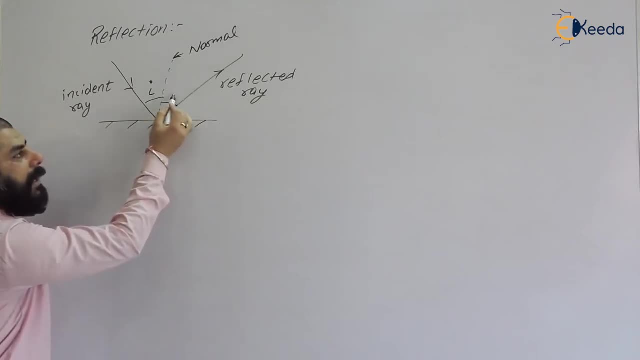 And the angle between normal and the reflected ray is called angle of reflection. So there are two laws in reflection. First law says that all the rays, that is, incident ray, normal ray and the reflected ray, all lie in the same plane. 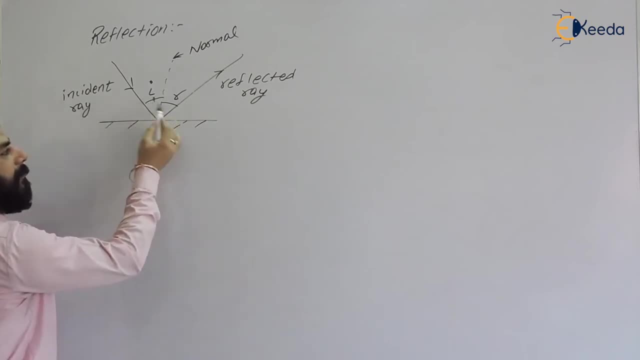 And second law says that angle of reflection that is equal to angle of reflection. So that is important for us, that angle of incidence is equal to angle of reflection. That is the second law of reflection, in which you- which is useful for us- that in a case of reflection, 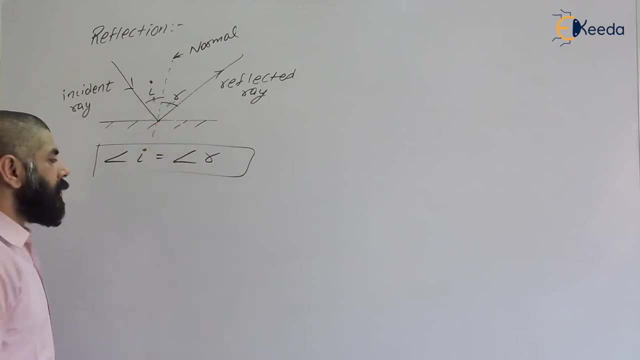 angle of incidence is equal to angle of reflection. So now we'll discuss about the reflection. See, when a light passes from one medium to another medium, it deviates from its path. That is called refraction. To understand that refraction phenomena, that why light deviates from its path, it will 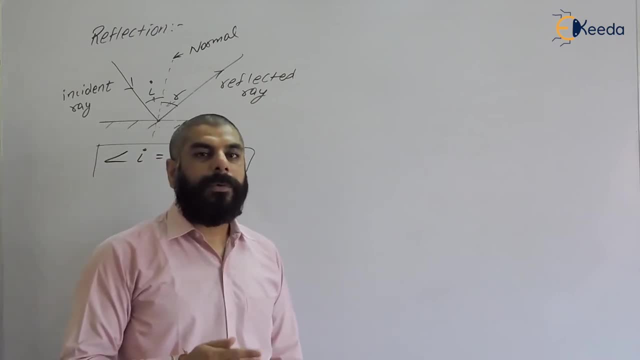 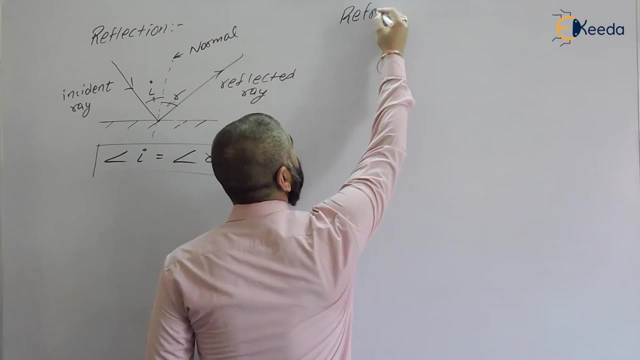 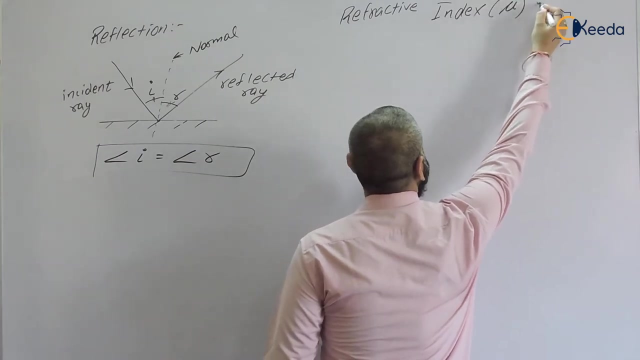 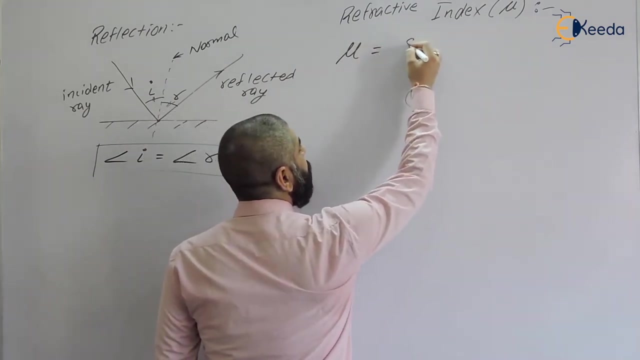 deviate towards the normal or away from the normal. So a medium is characterized by a term called refractive index. So let's see what is refractive index. Refractive index, Denoted by mu, This is defined as a. that refractive index of certain medium is defined as the speed. 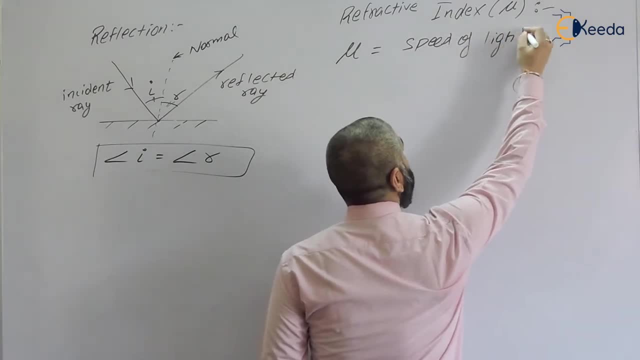 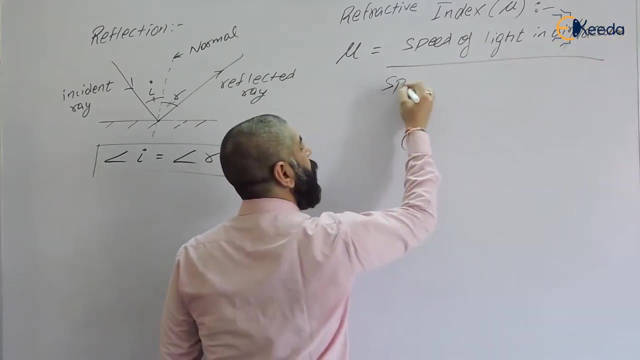 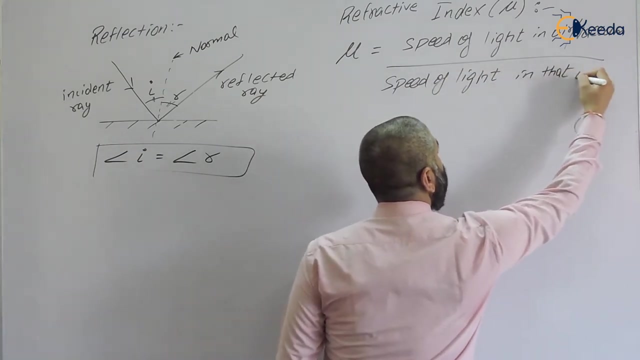 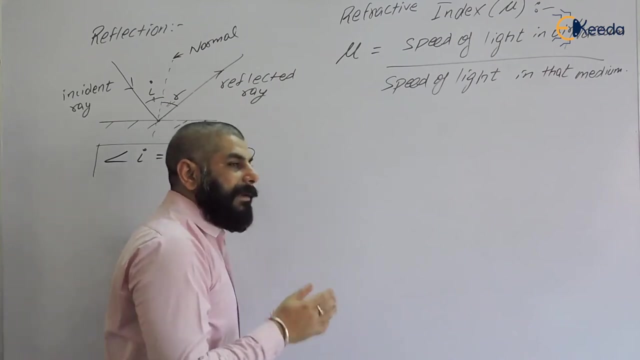 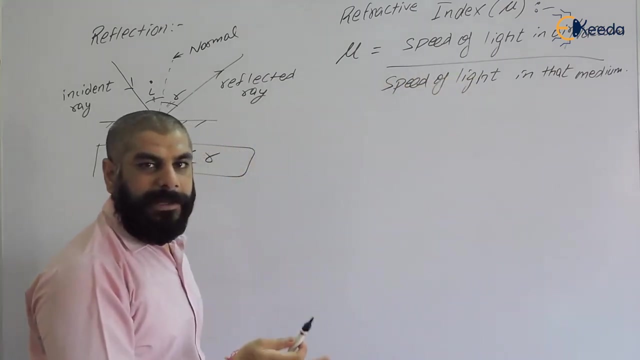 of light, speed of light in air or vacuum to speed of light in that medium. speed of light in that medium. Light has a different speed in different medium. See, if that medium has a higher refractive index, speed will be less, because speed of light in air is constant. 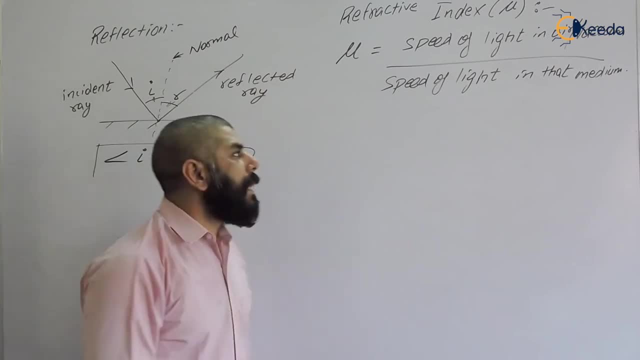 That is equal to 3 into 10, to the power, 8 meter per second. But speed of light in medium is different. Refractive index is inversely proportional to the speed of light in medium. So a medium which has high value of refractive index, the speed of light will be less. 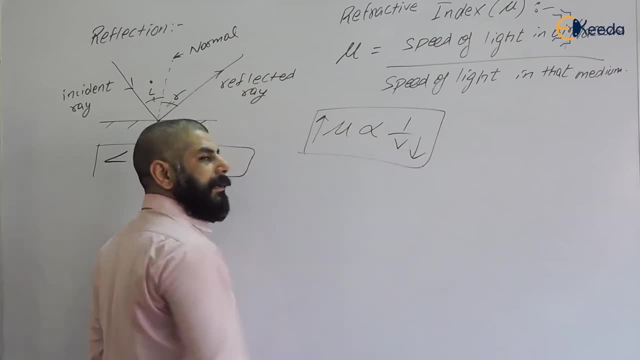 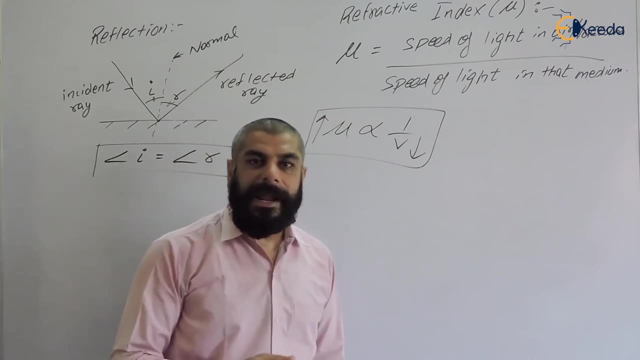 If refractive index is less, speed of light will be less. If refractive index is more, speed of light will be less in that medium. Then medium which is high refractive index, that is called denser medium, and the medium which is less, value refractive index. 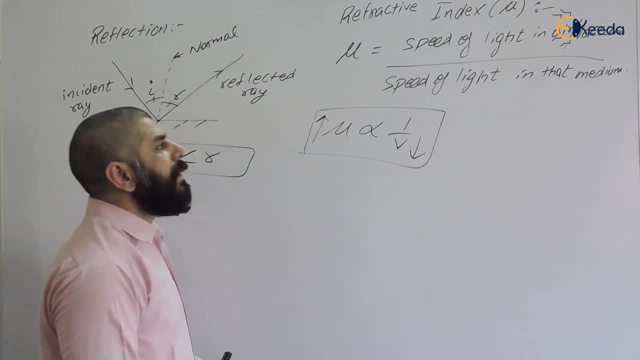 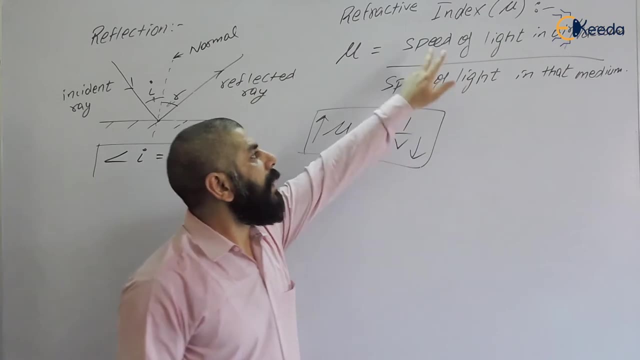 That is called rarer medium. see: maximum speed of light is in air, So maximum value of refractive index can be equal to what speed of light in air is maximum. it cannot go beyond light. It will be less than this. So medium. 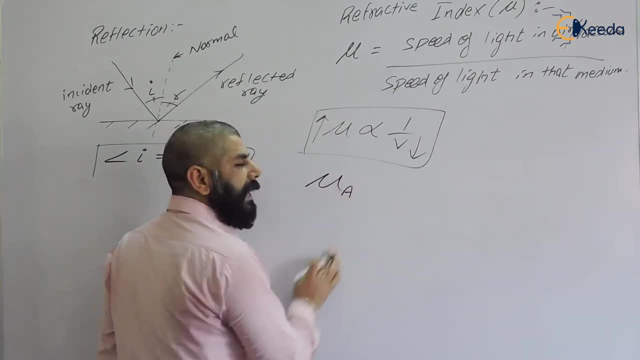 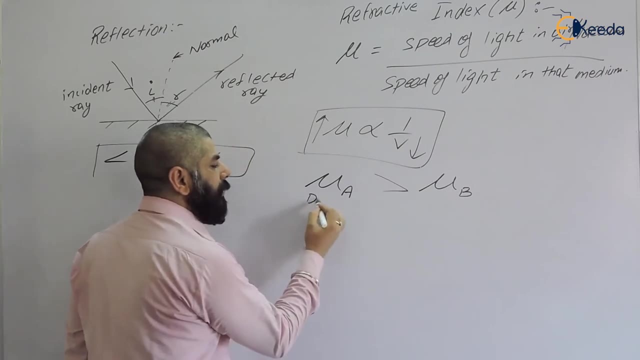 high value of refractive index. suppose we have two mediums: medium A has a refractive index mu A. medium B has a refractive index mu B. If mu A is greater than mu B, then this is called denser medium and this is called Rayleigh medium. So medium which has high. value of refractive index is therefore denser medium. Speed of light will be less in a denser medium- In case of Rayleigh medium- as compared to denser, so refractive index is less and the speed of light will be more compared to speed of light in denser. So now we will. 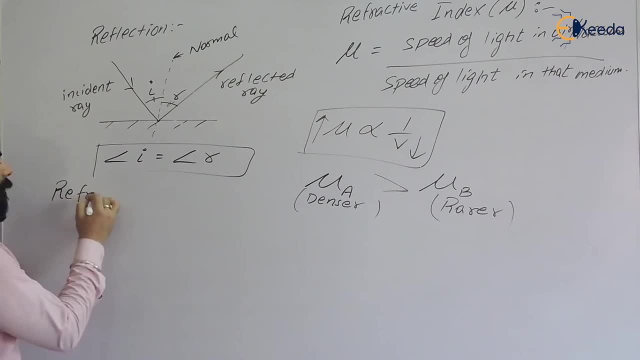 discuss about refraction. Refraction is the deviation of a light from its path when it travels from one medium to another medium. Suppose this was our incident ray, it will not go straight into the other medium. Suppose this is air, this is glass or some other medium. 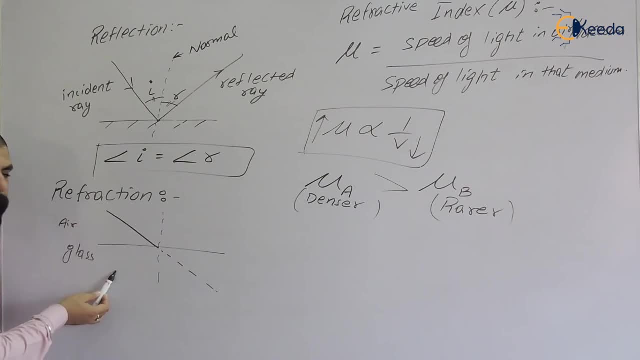 This is water or glass, one medium to another medium. We are considering medium 1 and medium 2.. So light is coming from this medium and enters into this medium, but it will not go straight. it will deviate away from the normal or towards the normal, If this medium is case. 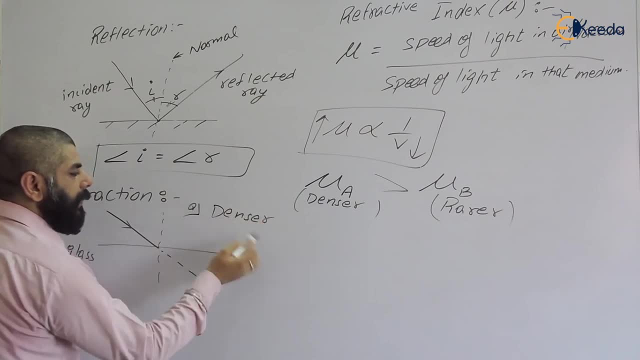 1, if this is denser, Case 1 means this is rayleigh medium and this is denser medium. Suppose this is medium 1, mu 1, this will deviate away from normal. This is medium 2.. Since 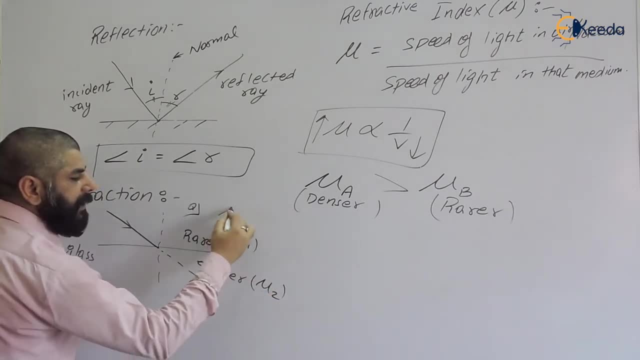 the refractive index mu2, so denser i am calling this. denser means mu2. refractive index of this medium is more than refractive index of medium one, so light will deviate. in case of denser medium, light bends towards the normal. this is our incident rate. 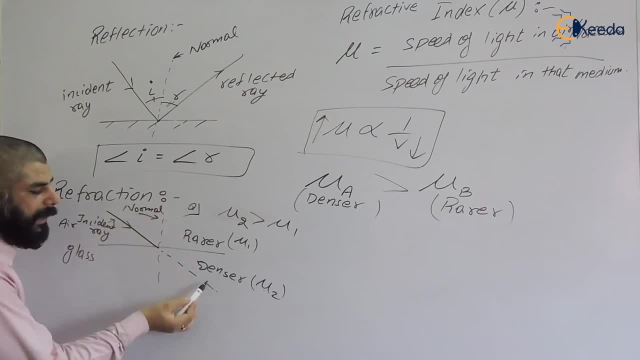 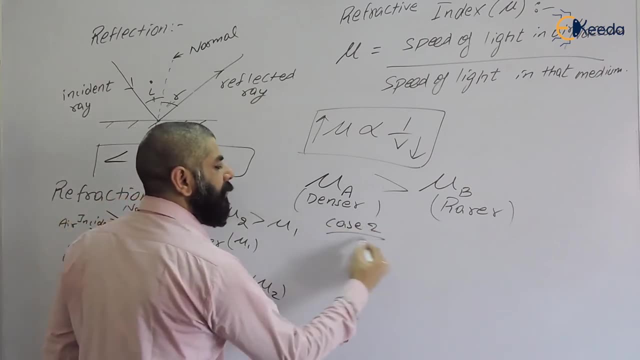 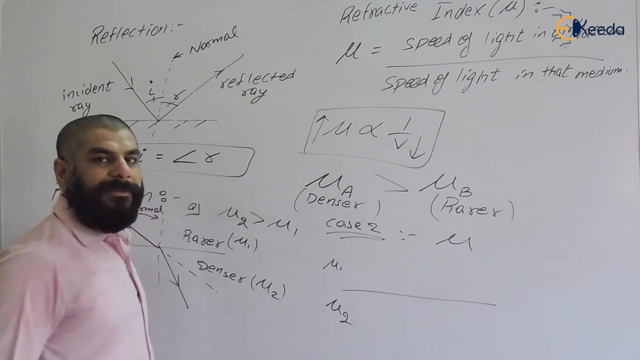 this is normal. so when light travels from barrier to tensor it deviates towards the normal. but case two: if light travels wrong, suppose this is medium one having refractive index mu2, this is medium two having refractive index mu2 when light propagates wrong. now, this time, first case, we saw that this 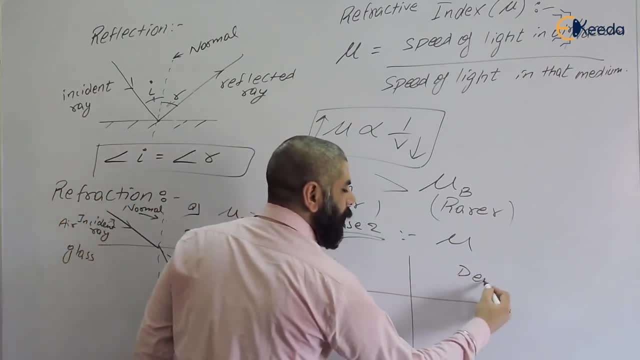 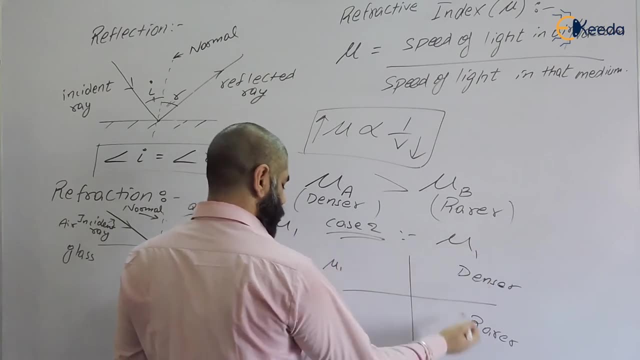 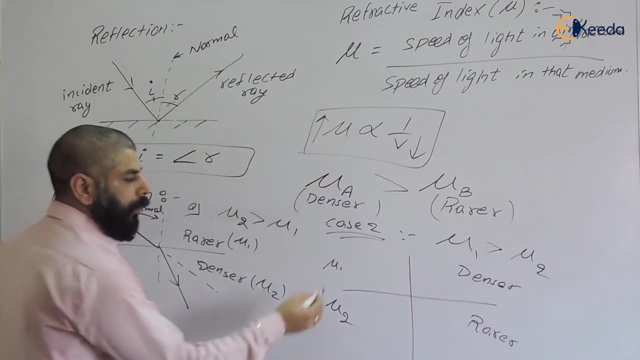 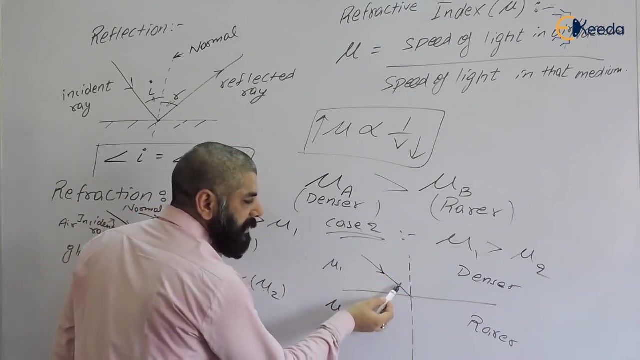 was there, this is dense. now reverse, this is denser and this is rarer. medium means refractive index of mu1 is more than refractive index of medium two. so when light travels, this is the normal right, this is our incident rate. when denser light travels from denser to there, it deviates from its 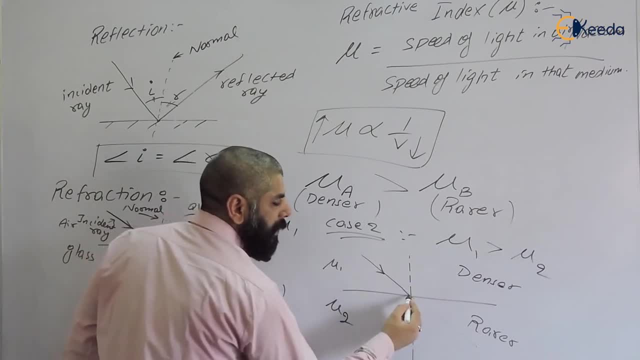 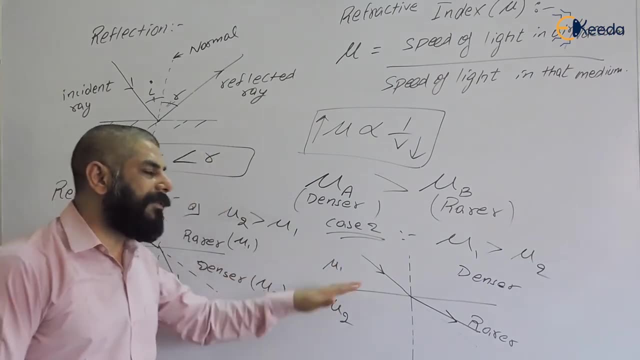 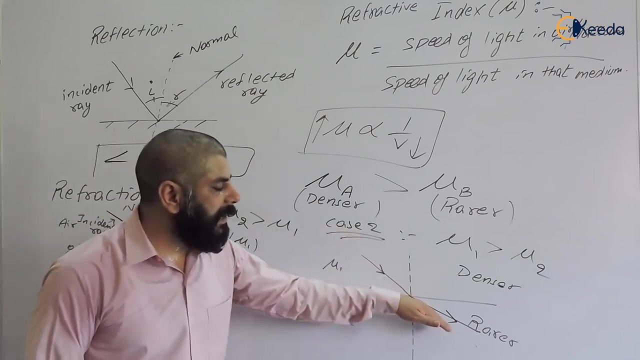 path. it will not go straight. it will bend away from the normal because the speed has a different light, has a different speed in different medium. so it deviates from its path. so when it moves from into denser medium it bends towards the normal. when it enters into rarer medium it bends away from the normal. so there is 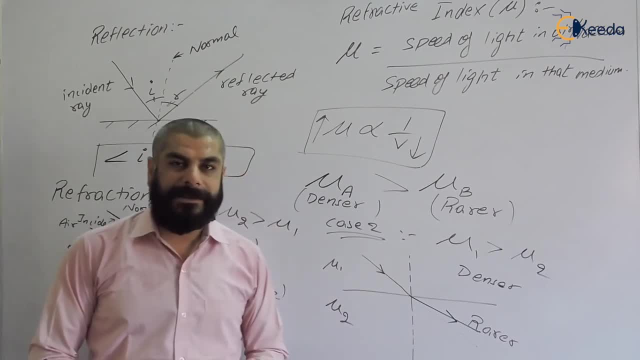 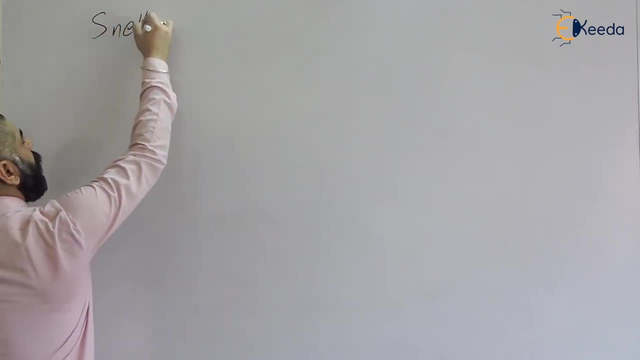 one law in reflection that is called snell's law. so what is this snell's law? let's discuss. so let's start snell's law. so what is snell's law? see, when a light enters from one medium to another medium, we saw that it will deviate from its path. this is our incident rate and this is our normal. 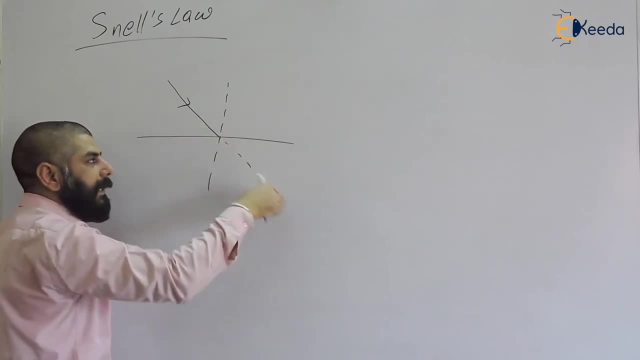 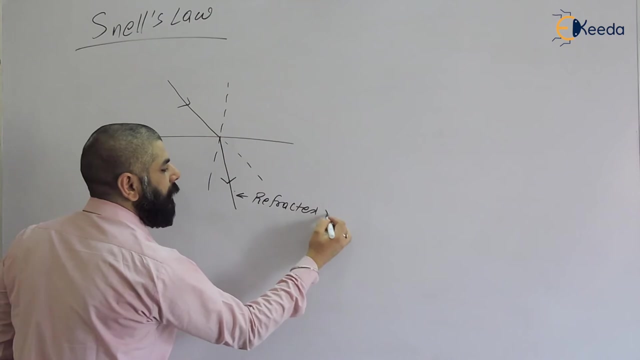 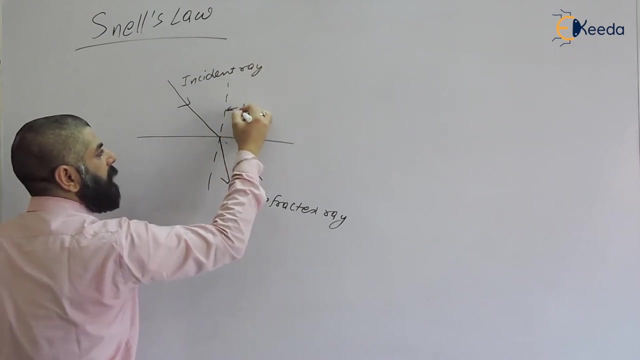 so it bends away from the normal or towards. it will not go straight path, it will deviate from its path. that this is called reflected rate, reflected rate and this is called incident rate. and the axis perpendicular that is called normal, perpendicular to the surface- see, this is medium one having reflective index, mu1. this 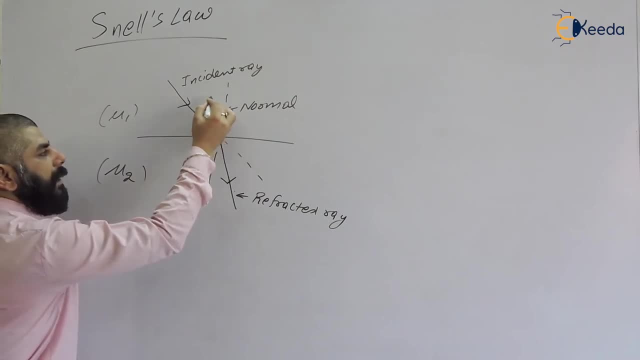 is the medium, two having effective index mu2. this is called angle of incidence, the angle between incident rate, normal, and this angle is called reflected angle, the angle between normal and a reflected rate. so what is snell's law? snell's law said that mu1 sine i sine of angle of incident. 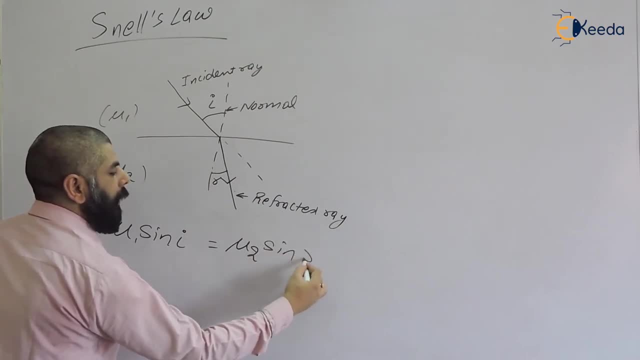 that is equal to a mu2 sine r. r is the angle of refraction. so mu1 sine i, that is equal to mu2 sine r. this is: mu1 is the refractive index of medium one. mu2 is the refractive index of medium 2 to mu 1 sin i. that is equal to mu 2 sin r. See, there is one more term that is called 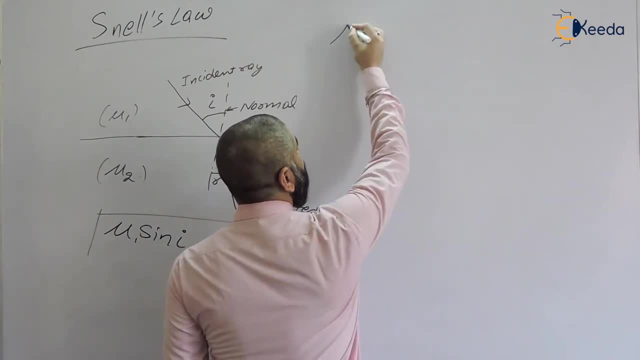 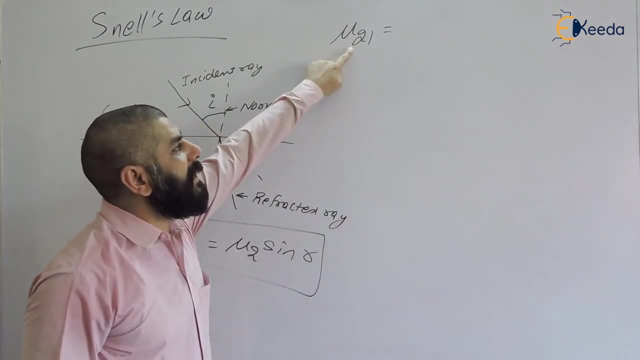 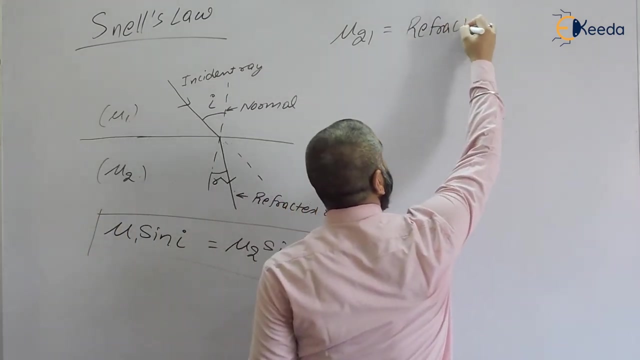 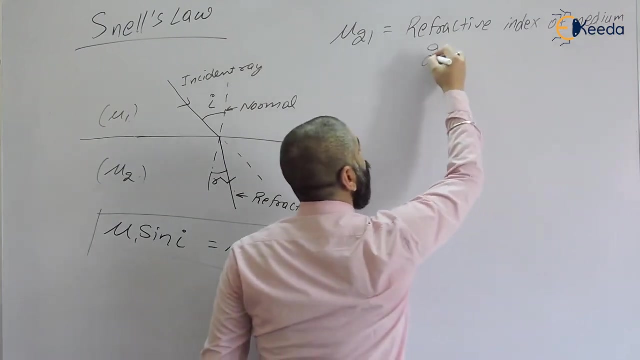 relative refractive index. What is relative refractive index? This term 2 raised to 1, this is read as refractive index of medium 2 with respect to medium 1.. So this is defined as refractive index of refractive index of medium 2 with respect to medium with respect. 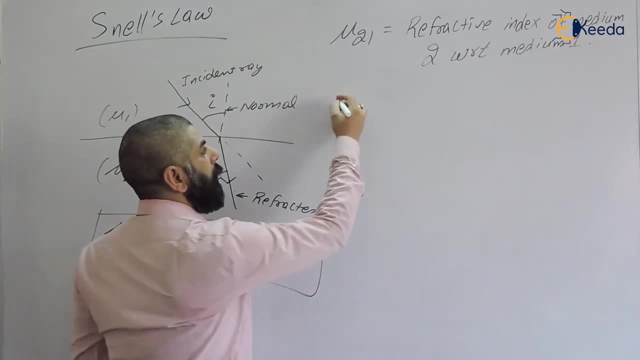 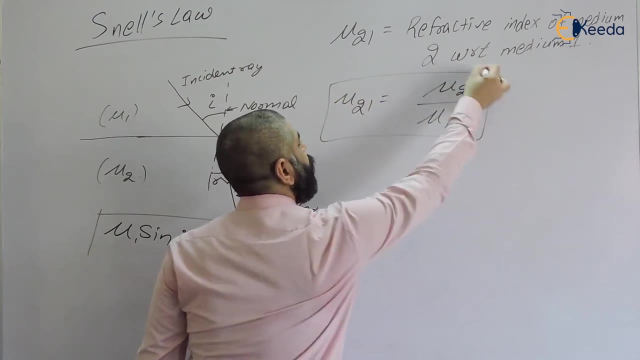 to refractive index of medium 1.. So this is defined as wavelength index of medium 2 divided by reflective index of medium 1.. right, So it is read as a reflective index of medium 2 with respect to medium 1.. 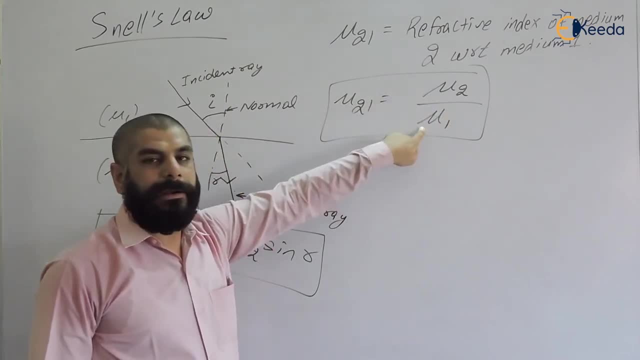 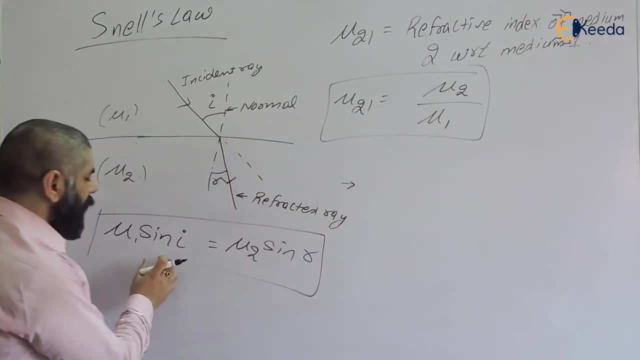 So refractive index of medium 2 with respect to air divided by refractive index of medium 1 with respect to air. So we will derive one formula From Snell's law. we saw that mu 1 by mu 2, that is equal to me. 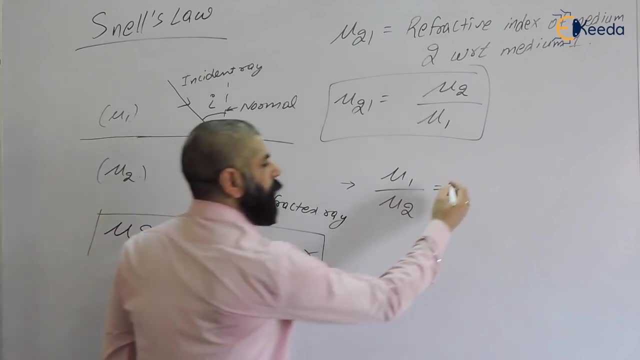 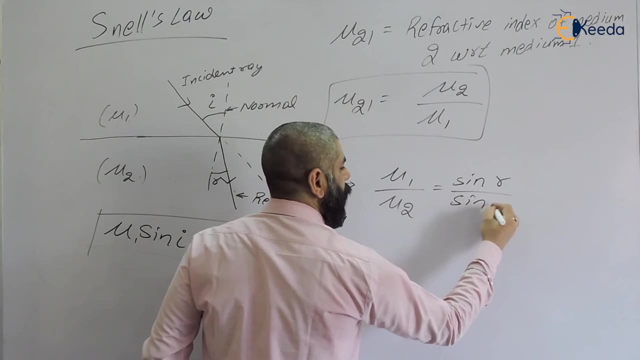 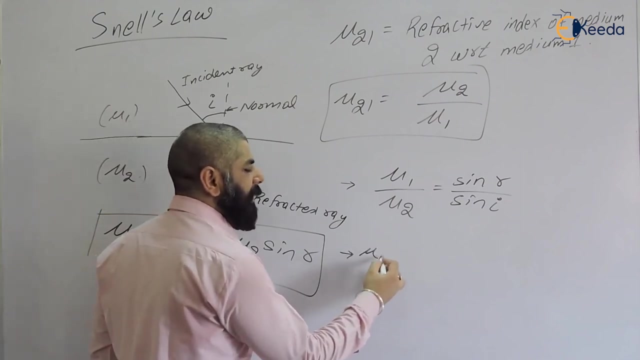 See, this will come denominator, so this will go here. That is equal to sin r by sin i. Now, when we define the definition of refractive index, Refractive index is defined as the speed of light in air to the speed of light in vacuum. 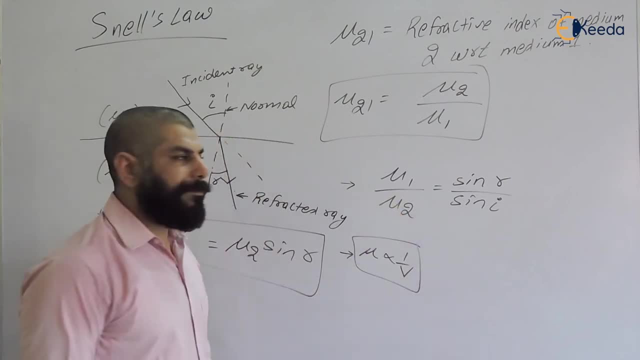 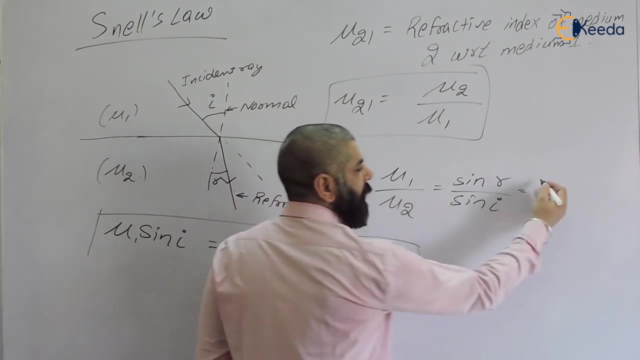 Means refractive index is inversely proportional to velocity. So here it will come out to be: If we divide these two: refractive index is inversely proportional to velocity. So this will become v2 by v1.. v2 is the velocity in medium 2.. 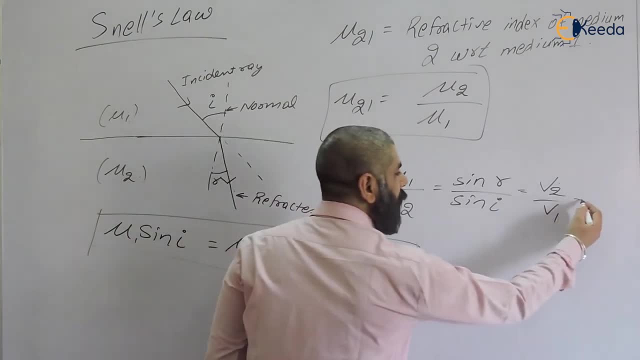 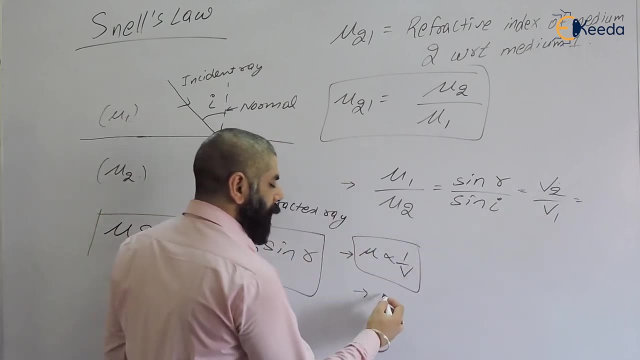 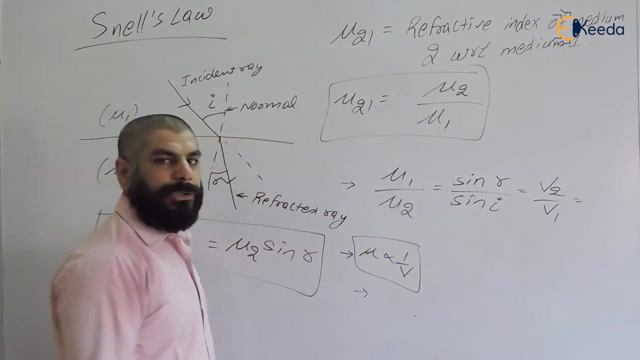 v1 is the velocity in medium 1. Now, from relation that, see what is the relation between velocity and a wavelength? See mu. what is c by lambda? mu equal to c by lambda? Velocity is directly proportional to wavelength mu equal to c by lambda. 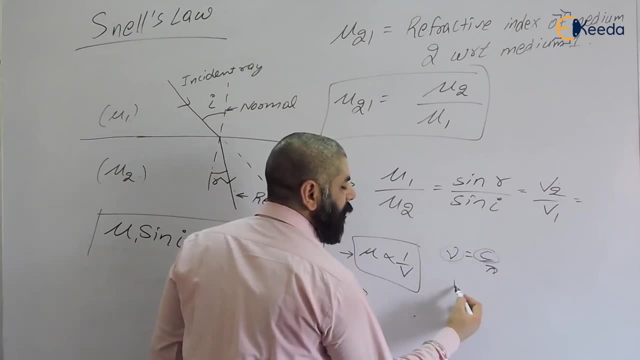 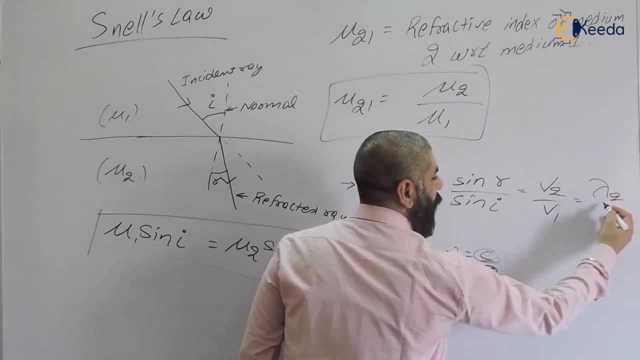 If frequency is constant at a speed, that is, speed is or the velocity is directly proportional to lambda. So this velocity, v2 by v1, that will come out to be Lambda 2.. V2 by lambda 1.. 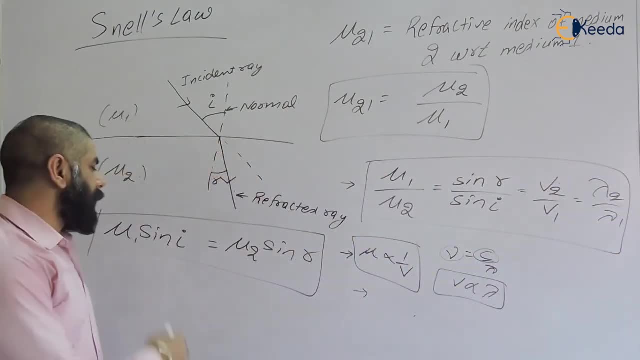 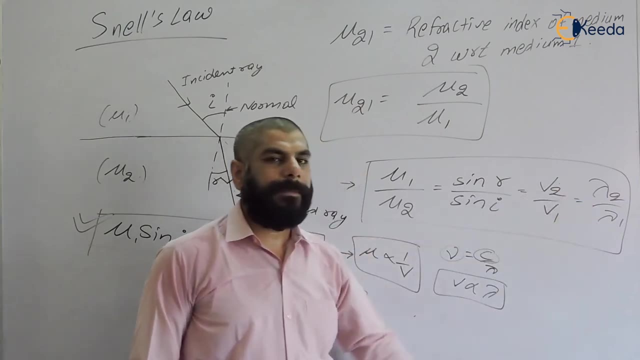 So we will use this formula in case of sorting the numerical. So this is the Snell's law, And also we will use this relation: mu 1 by mu 2, that is equal to v2 by v1, equal to lambda 2 by lambda 1..